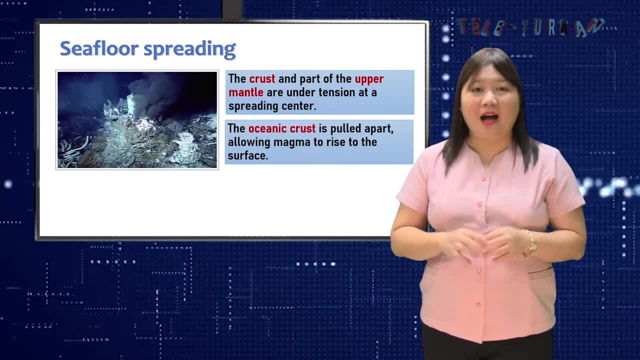 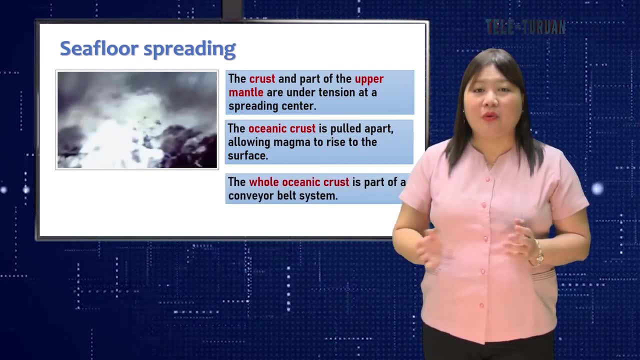 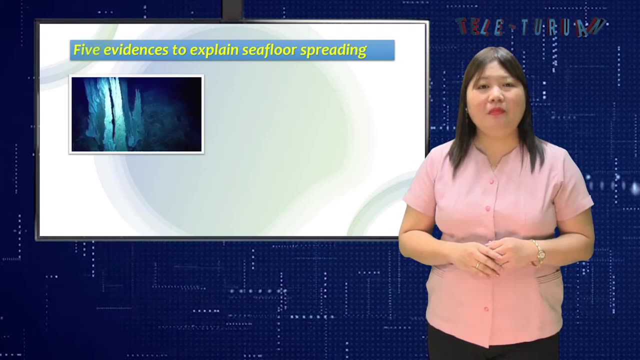 seafloor. Thus the ocean crust is pulled apart, allowing magma to rise to the surface, and the whole oceanic crust is part of a conveyor belt system, rising up at the mid-ocean reaches and eventually sinking down at the oceanic trenches. We can explain seafloor spreading by considering: 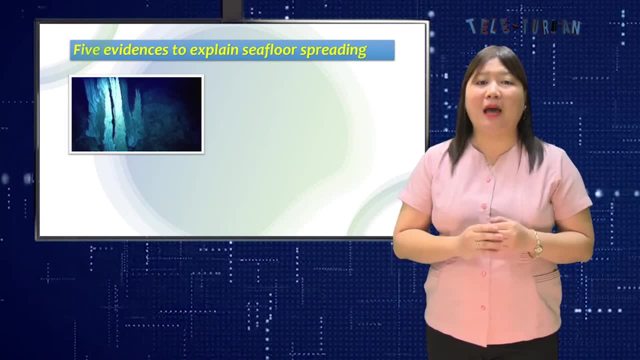 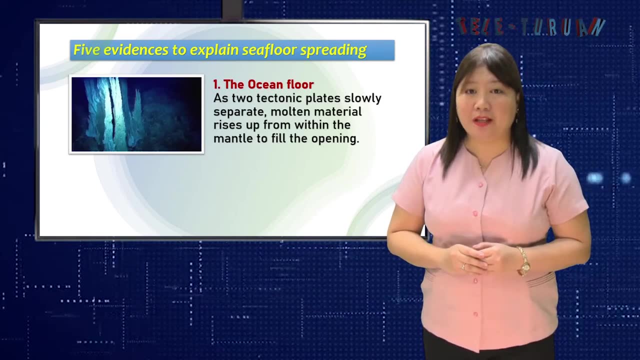 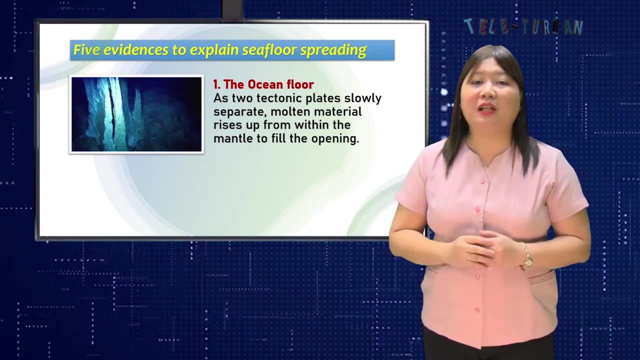 the usual process at work at divergent plate boundaries, which evidently describes how seafloor spreads. The ocean floor can explain the occurrence of seafloor spreading. As two tectonic plates slowly separate, molten material rises up from within the mantle to fill the opening In this way. 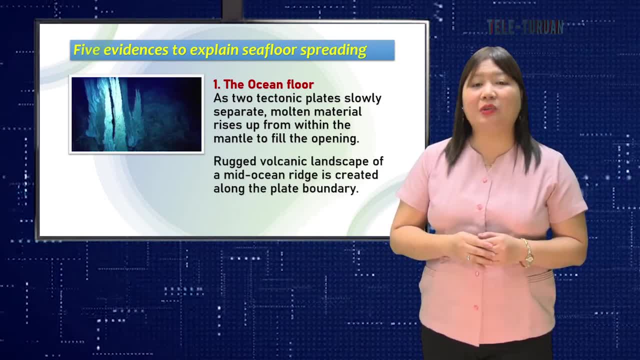 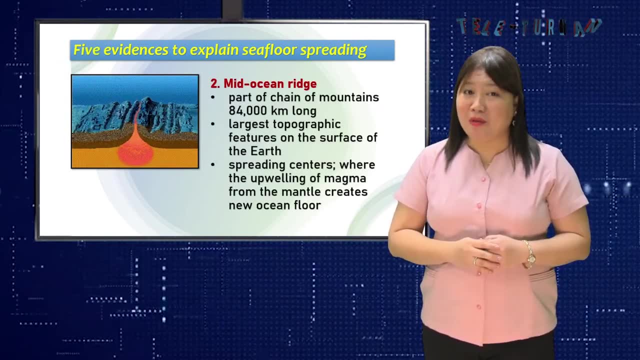 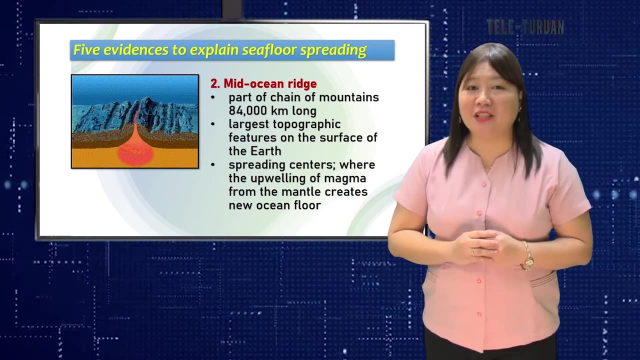 the rugged volcanic landscape of a mid-ocean ridge is created along the plate boundary. Second is the mid-ocean ridge. Remember that mid-Atlantic ridge is the longest mountain chain on earth. Mid-ocean ridges are parts of chain of mountains some 84,000 kilometers long and are the largest. 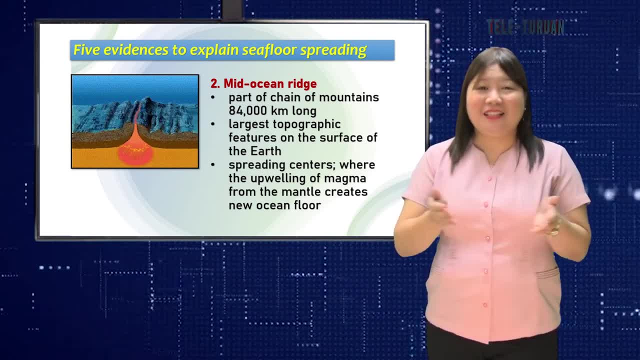 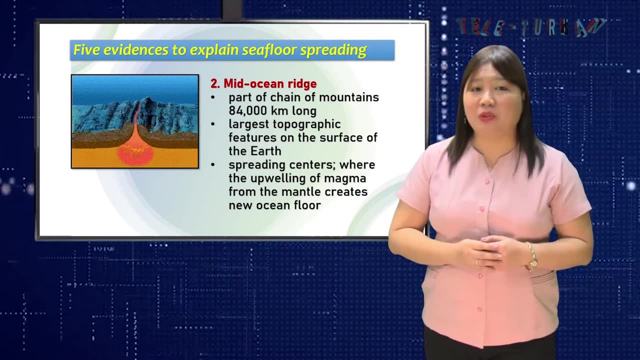 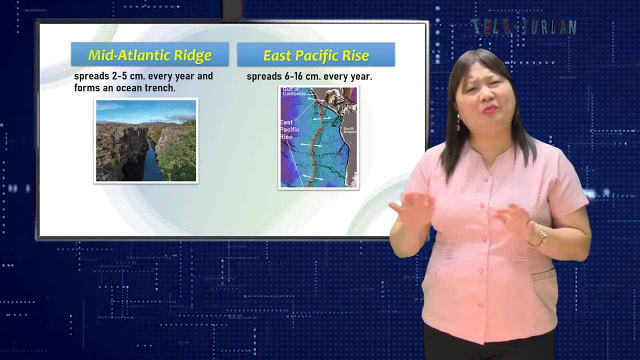 topographic features. on the surface of the earth, These ridges are spreading centers or divergent plate boundaries, where the upwelling of magma from the mantle creates new ocean floor. The mid-Atlantic ridge, for instance, is a slow spreading center. It spreads 2 to 5 centimeters every year. 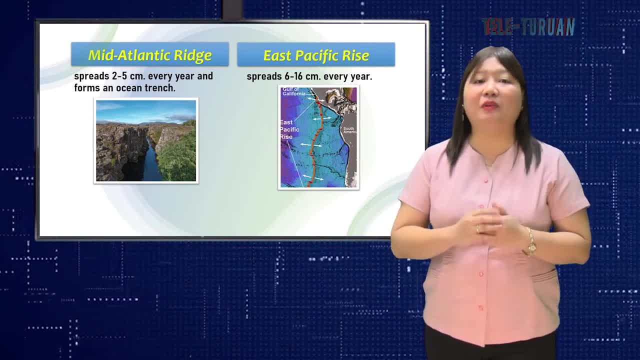 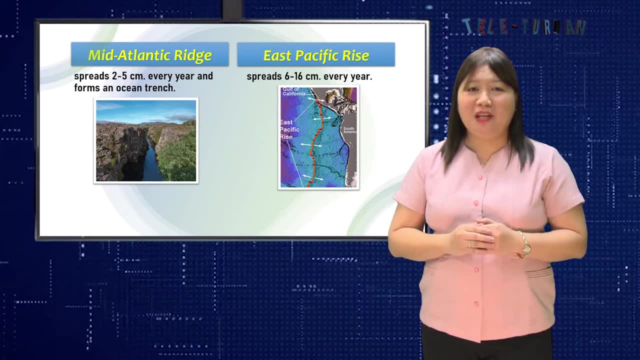 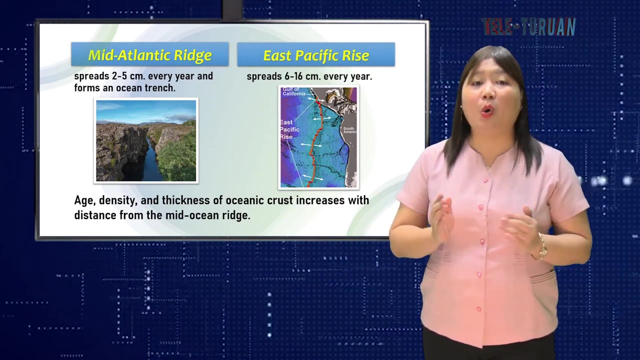 It forms an ocean trench, whereas the East Pacific rise is a fast spreading center. It spreads about 6 to 16 centimeters every year. Take note that age density and thickness of oceanic crust increases with distance from the mid-ocean ridge. Third, the evidence of deep sea trench. 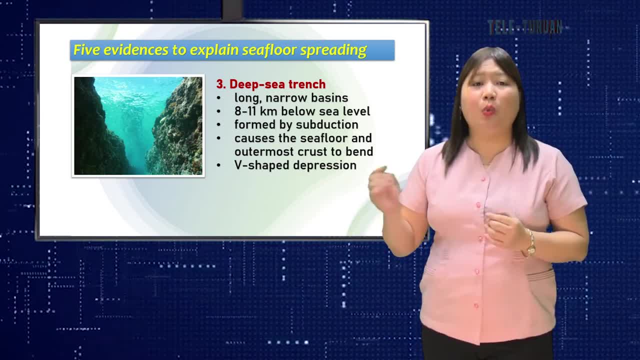 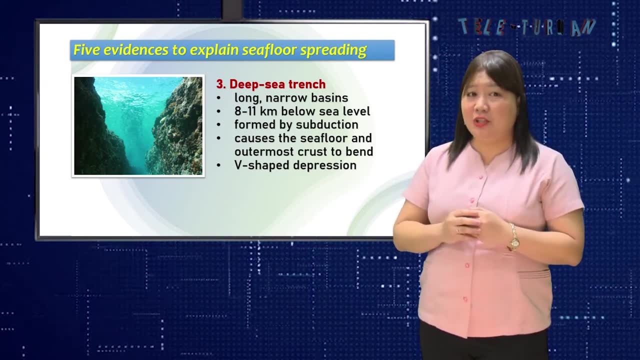 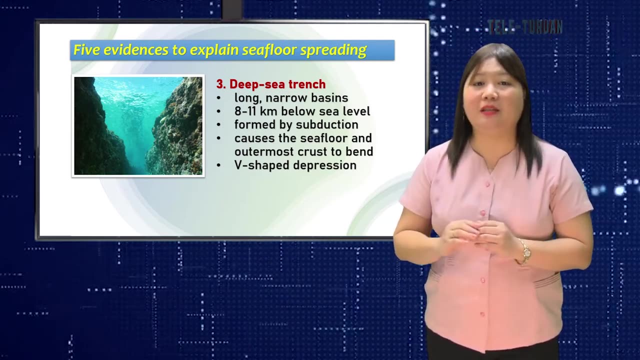 Deep sea trenches are long, narrow basins which extend 8 to 11 kilometers. Trenches are formed by subduction in which two or more tectonic plates converge. An older, denser plate is pushed beneath the lighter plate and dipped into the mantle, causing the 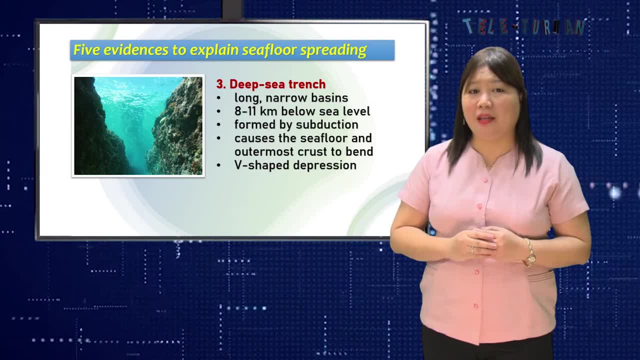 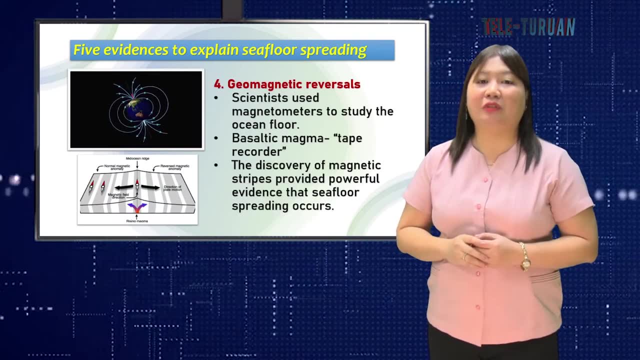 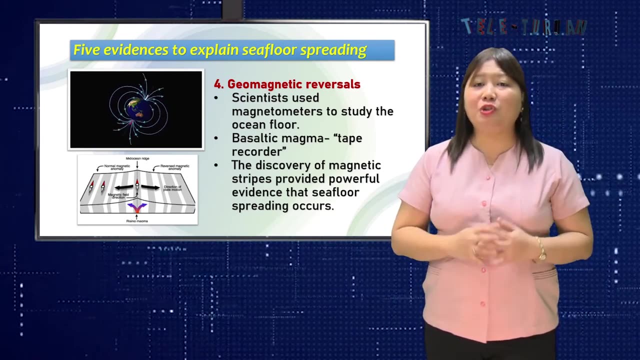 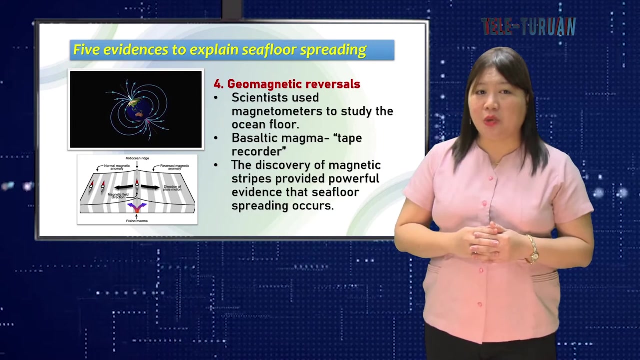 seafloor and outermost crust to bend and form a steep v-shaped depression. Fourth is the geomagnetic reversals, When research scientists use magnetometers to study the ocean floor. measurements of magnetic variation showed that alternating dance of rocks recording normal and reverse polarity were arranged symmetrically about mid-ocean ridges. 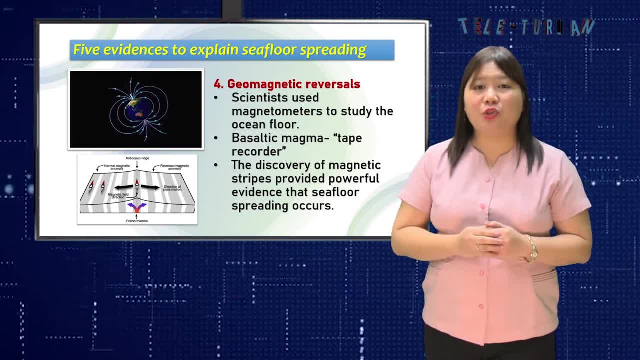 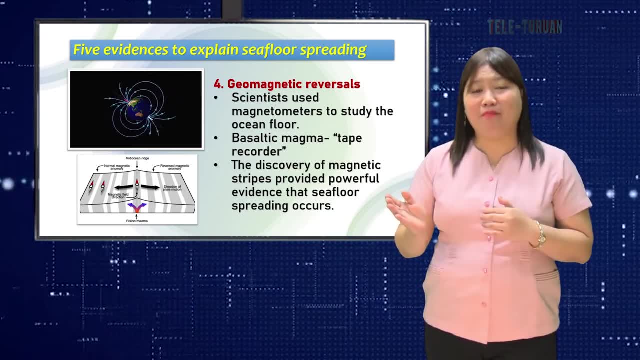 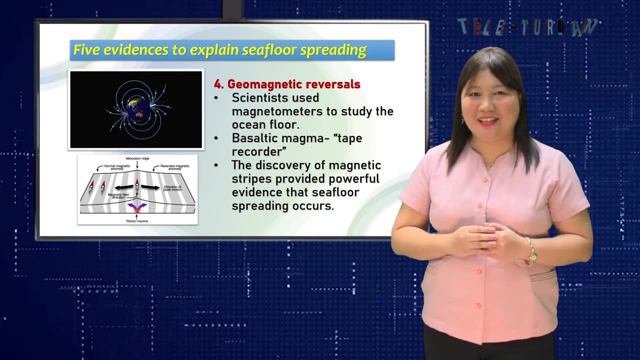 Basaltic magma forming at mid-ocean ridges serves as a kind of tape recorder recording the Earth's magnetic field as it reverses through time. The discovery of such magnetic stripes provided powerful evidence that seafloor spreading occurs. Fifth, the age of the seafloor discloses seafloor spreading. Scientists noticed that from the ridge. crests, sediment becomes older and the seafloor becomes thicker. Since the oldest ocean crust is so much younger than the oldest continental crusts, scientists realized that something was happening to the older seafloor. The oldest known ocean floor is dated at about 200 million years ago. 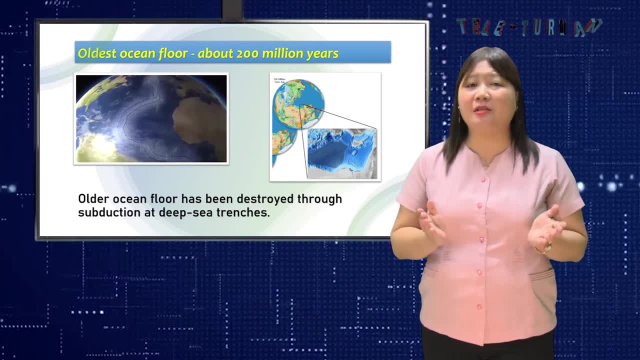 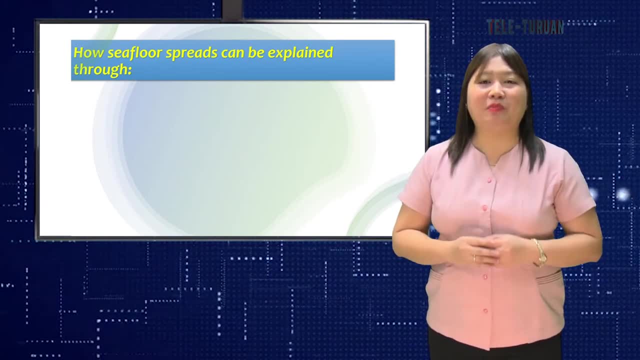 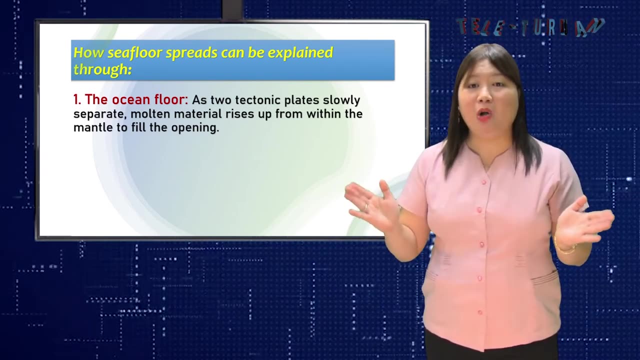 The median age is estimated to be about 1.5 billion years, indicating that older ocean floor has been destroyed through subduction at deep sea trenches. To sum up how seafloor spreads can be explained through one: the ocean floor as two tectonic plates slowly separate molten material prices up from 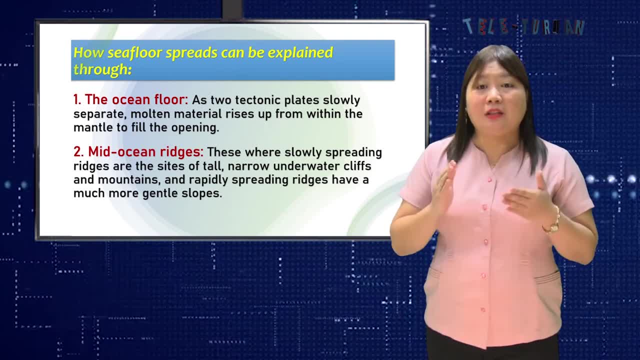 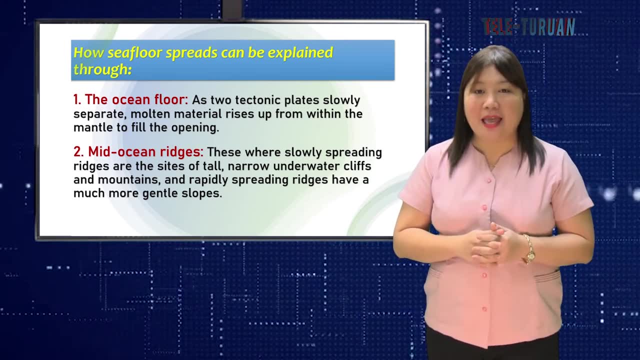 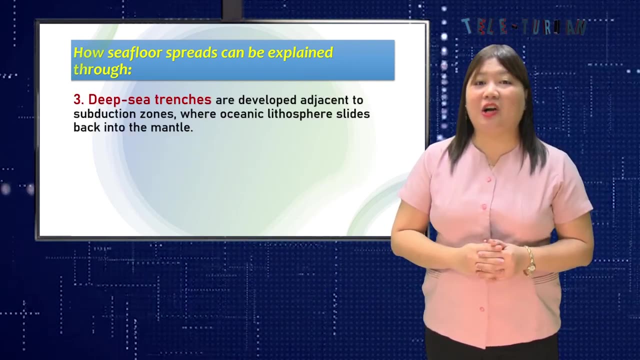 within the metal to fill the opening to mid-ocean bridges. This were slowly spreading ridges are the narrow underwater cliffs and mountains, and rapidly spreading ridges have much more gentle slopes. Three deep sea trenches are developed adjacent to subduction zones where oceanic lithosphere 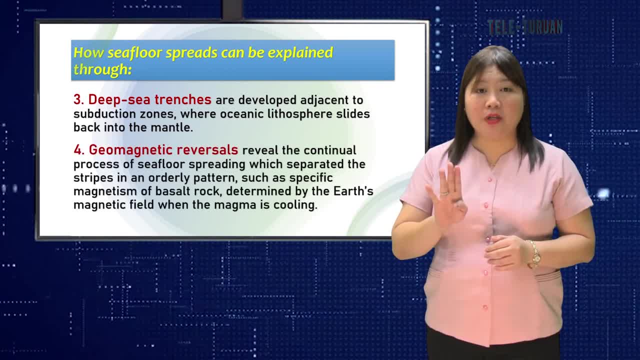 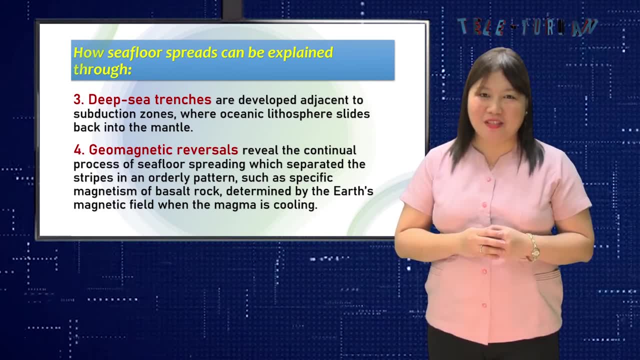 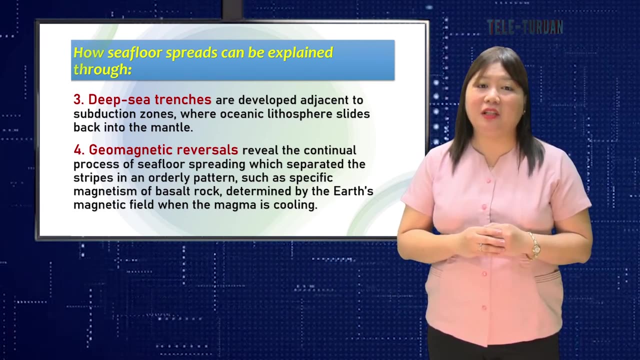 is sliced back into the mantle. Number four geomagnetic reversals reveal the continual process of seafloor spreading, which separated the stripes in an orderly pattern, such as a specific magnetism of basalt rock determined by the earth's magnetic field when the magma is cooling. 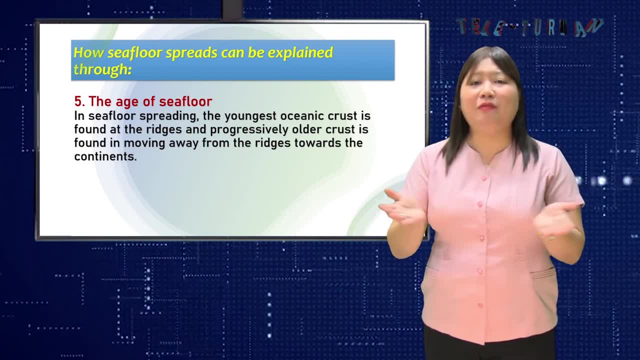 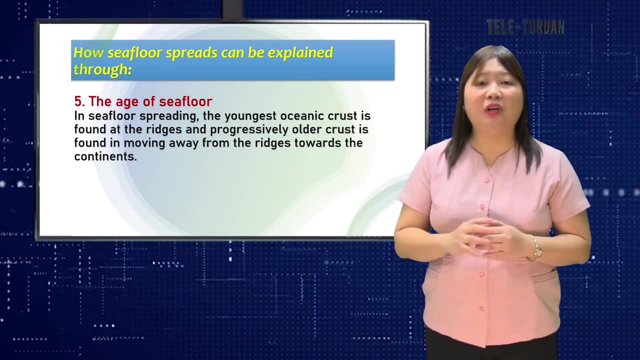 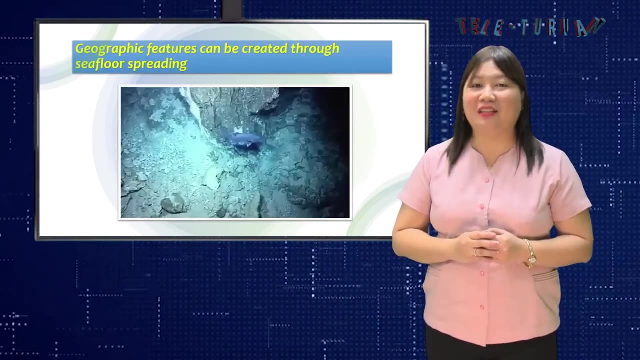 Number five: the age of seafloor. In seafloor spreading, the youngest oceanic crust is found at the ridges and progressively older crust is found in moving away from the ridges towards the continents. In the end, new geographic features can be created through seafloor spreading.